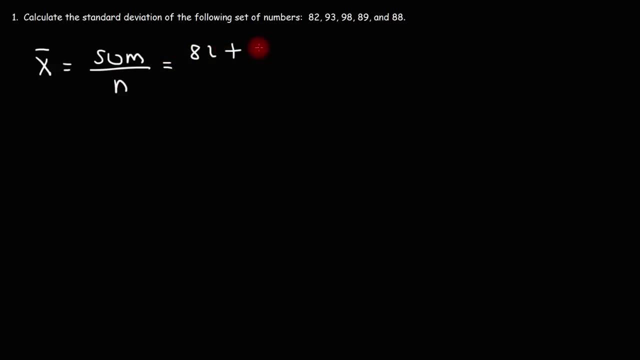 So we're going to add up the five numbers that we have: 82 plus 93 plus 98 plus 89 plus 88.. And since we have five numbers, we are going to divide this by five, So 82 plus 93 plus 98 plus 89 plus 88. 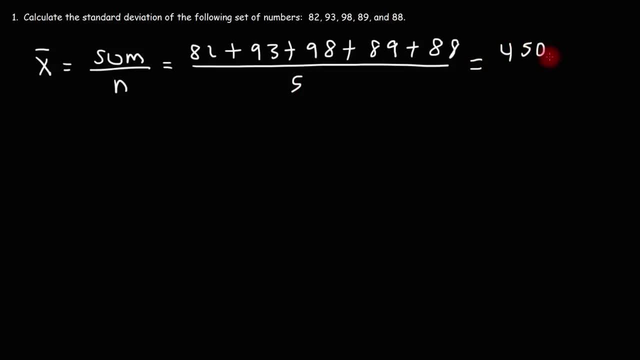 That gives us a sum of 450.. Now let's divide that by five. 45 divided by five is nine, And if we add a zero, that gives us an average of 90.. So that is our sample mean. Now the formula that we're going to use to calculate the standard deviation is this formula: 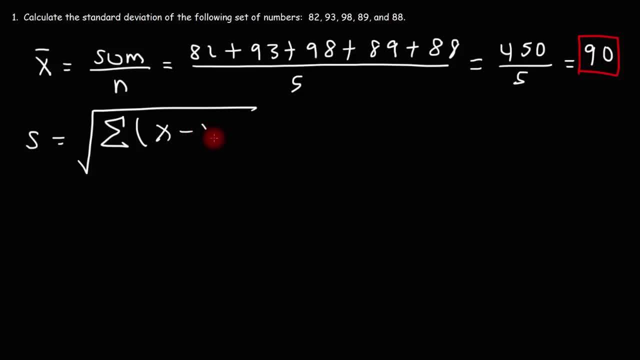 So we're going to take the difference of each x value and the mean, And then we're going to square those differences and take the sum of those squares And then we're going to divide it by n minus one. So let me show you how to do that. 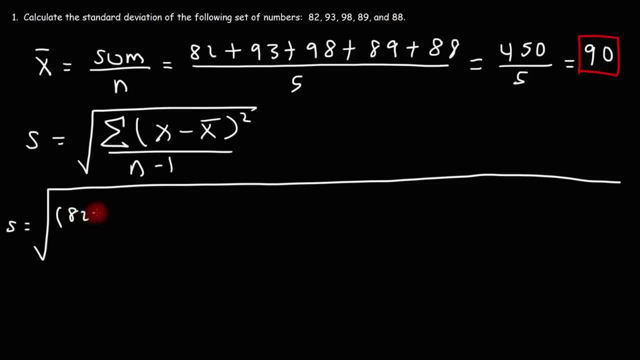 So the first number is: We're going to subtract that from the mean, which is 90.. And then square it. The next number is 93.. We're going to subtract it from the mean and then square it. The mean is 90.. 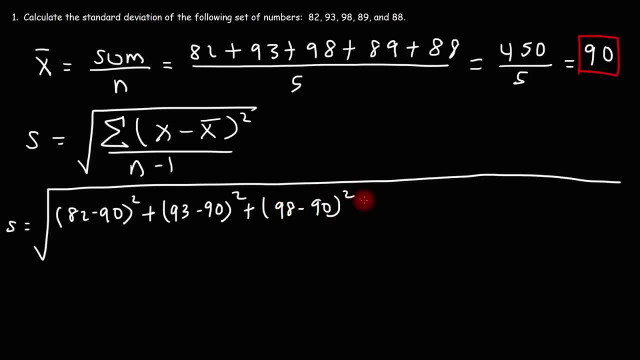 And then it's going to be 98 minus 90.. And then we're going to keep doing this until it's finished. So n is five, n minus one is going to be five minus one or four. Now let's do this one step at a time. 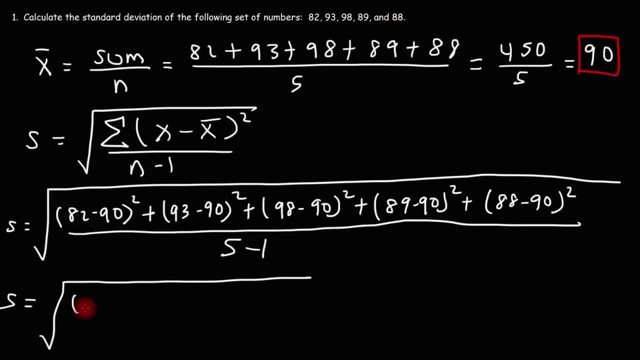 82 minus 90 is negative eight. So this is going to be negative eight squared, But once you square it the negative sign won't matter, And then it's going to be plus three squared: 98 minus 90 is eight. 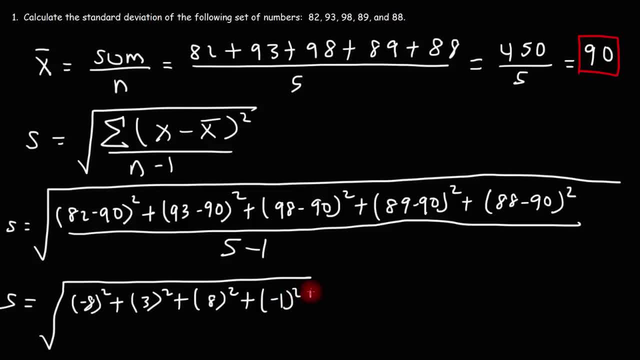 89 minus 90 is negative one, And so forth, And then divide it by four. So go ahead and type this in, So we have eight squared plus three squared Plus eight squared Plus one squared Plus two squared, So that adds up to 142.. 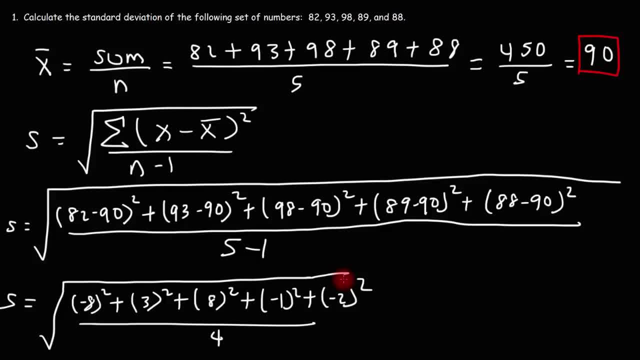 Divide that by four And then take the square root of that result, And so you should get a standard deviation of 5.958.. So this is the answer. Now let's try another example. but Let's try another example, but. 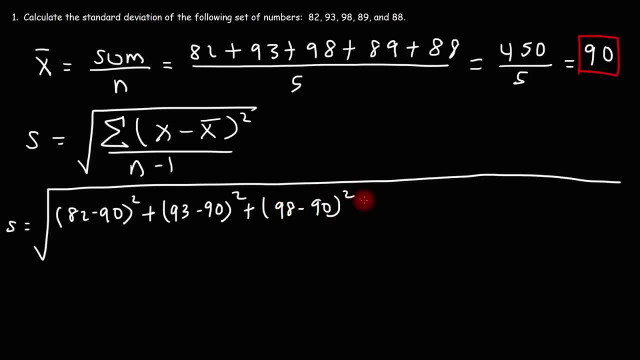 And then it's going to be 98 minus 90.. And then we're going to keep doing this until it's finished. So n is five, n minus one is going to be five minus one or four. Now let's do this one step at a time. 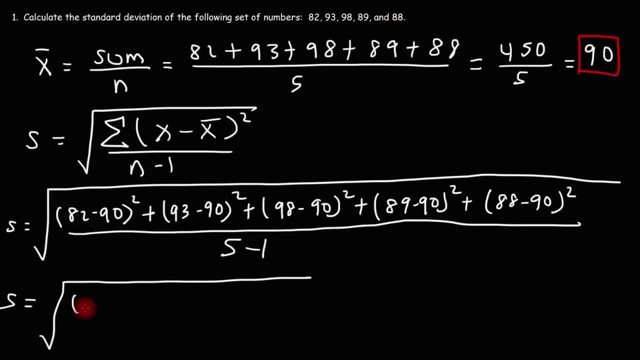 82 minus 90 is negative eight. So this is going to be negative eight squared, But once you square it the negative sign won't matter, And then it's going to be plus three squared: 98 minus 90 is eight. 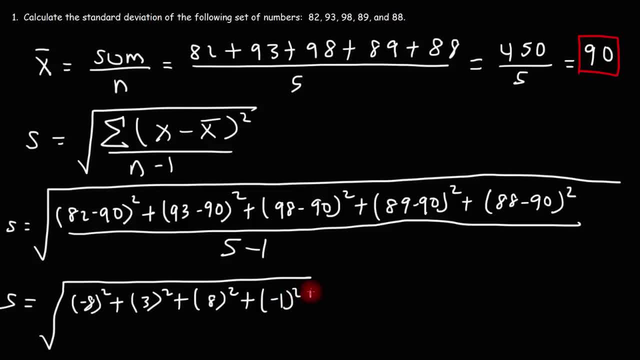 89 minus 90 is negative one, And so forth, And then divide it by four. So go ahead and type this in, So we have eight squared plus three squared Plus eight squared Plus one squared Plus two squared, So that adds up to 142.. 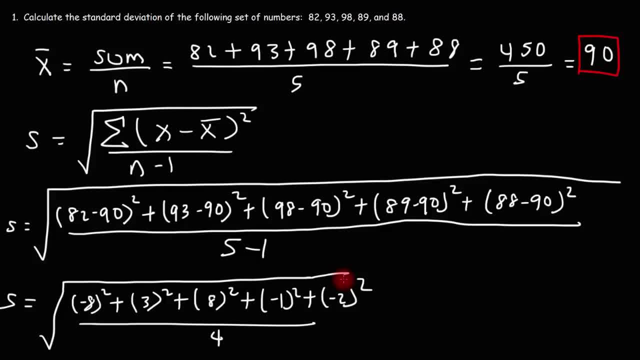 Divide that by four And then take the square root of that result, And so you should get a standard deviation of 5.958.. So this is the answer. Now let's try another example. but Let's try another example, but. 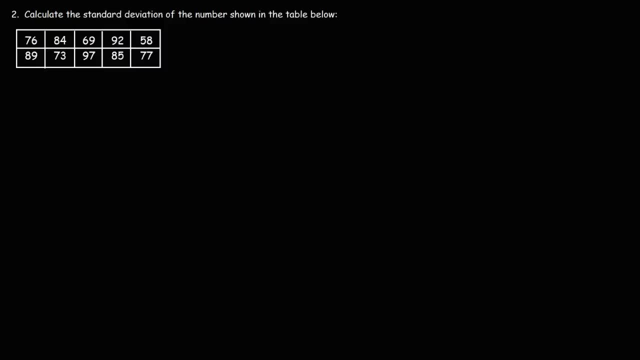 One with more numbers involved. So go ahead and try this. Calculate the standard deviation of The numbers- I forgot the S there- The numbers shown in the table below. Feel free to pause the video and try it. So let's begin by calculating the sample mean. 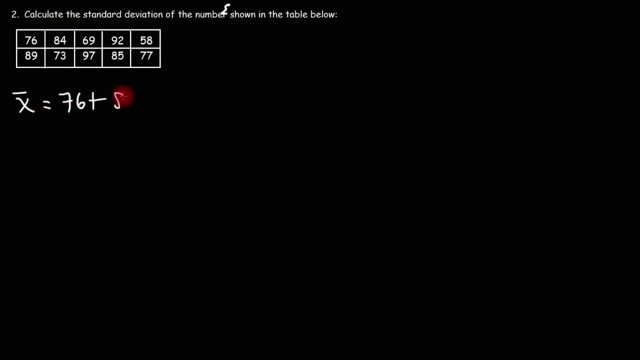 So let's take the sum of all the numbers. So we have 76 plus 84. Plus 69. Plus 92. Plus 58. Plus 89. And so forth. So we're going to take the sum of all of these numbers. 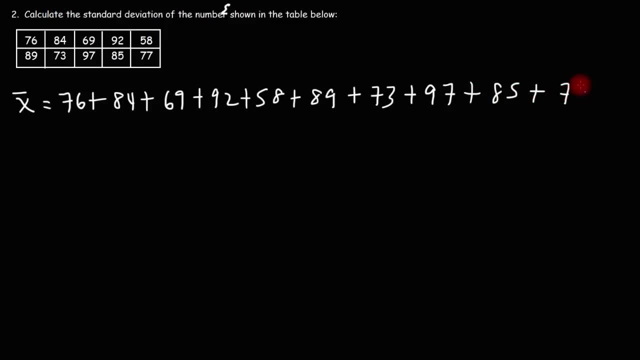 And then we're going to divide it by the size of the sample. And then we're going to divide it by the size of the sample. So in that sample we have 10 numbers. So N is 10.. 76 plus 84 plus 69.. 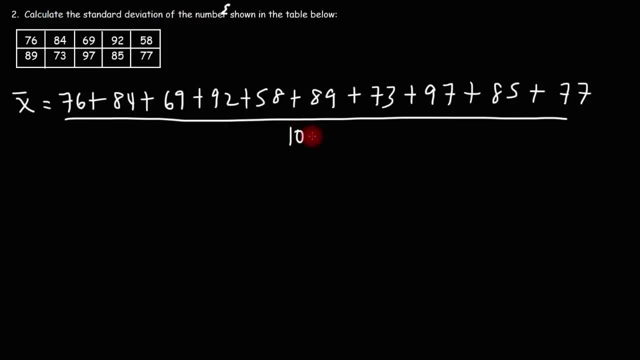 76 plus 84 plus 69. Plus 82. Plus 82. Plus 58. Plus 89. Plus 90. Plus 90.. Let me try that again. I think I did that wrong. So the sum of those 10 numbers is 800.. 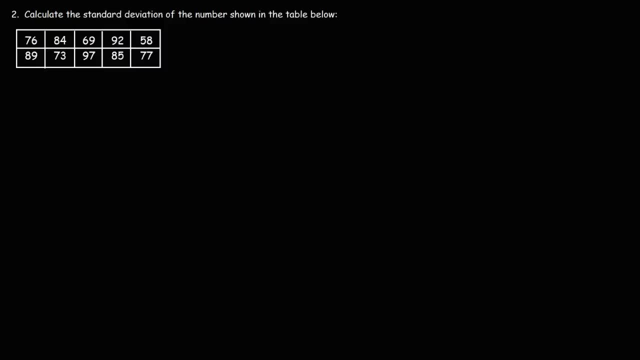 One with more numbers involved. So go ahead and try this. Calculate the standard deviation of The numbers- I forgot the S there- The numbers shown in the table below. Feel free to pause the video and try it. So let's begin by calculating the sample mean. 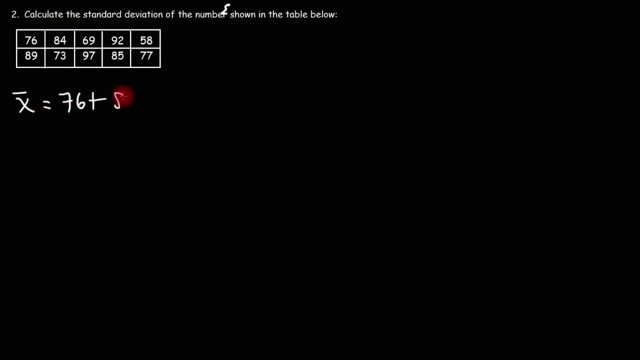 So let's take the sum of all the numbers. So we have 76 plus 84. Plus 69. Plus 92. Plus 58. Plus 89. And so forth. So we're going to take the sum of all of these numbers. 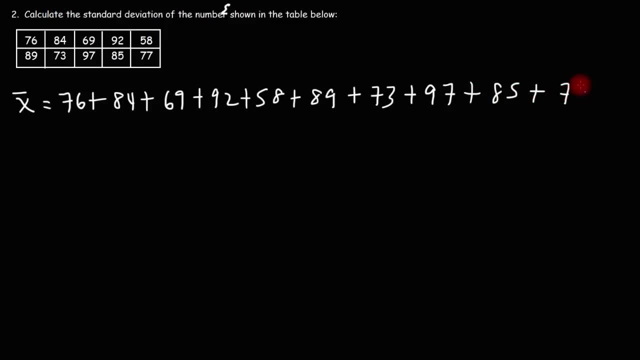 And then we're going to divide it by the size of the sample. And then we're going to divide it by the size of the sample. So in that sample we have 10 numbers. So N is 10.. 76 plus 84 plus 69.. 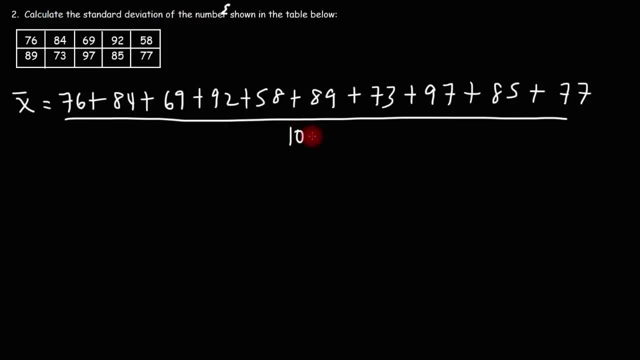 76 plus 84 plus 69. Plus 82. Plus 82. Plus 58. Plus 89. Plus 90. Plus 90.. Let me try that again. I think I did that wrong. So the sum of those 10 numbers is 800.. 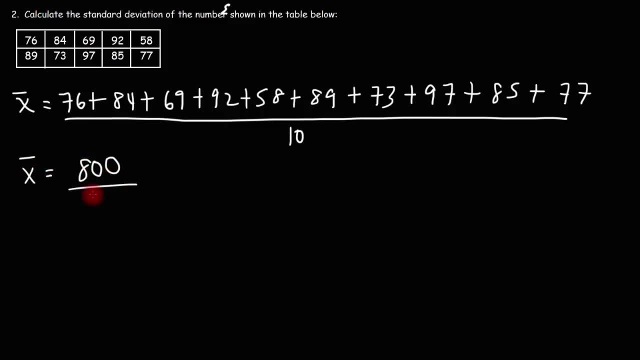 So the sum of those 10 numbers is 800. And if we divide it by 10, this will give us an average of 80. So that's the sample mean. Now let's calculate the standard deviation of the sample. So let's use the same formula that we. 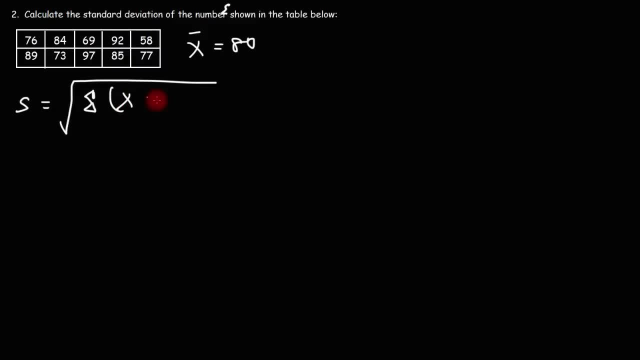 used earlier. So it's going to be the first number, 76.. Minus the mean, Which is 80.. And then squared, And then it's going to be the next one, Which is 84.. Minus the mean. 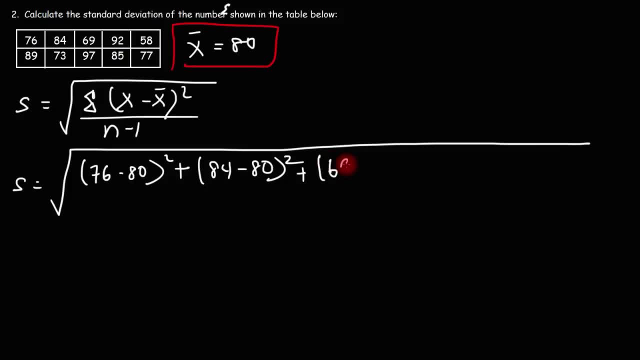 And then don't forget to square it. And then we need to do this for all of the numbers. So the last one is going to be 77 minus 80 squared, And then divide it by N minus 1. So we have 10 numbers. 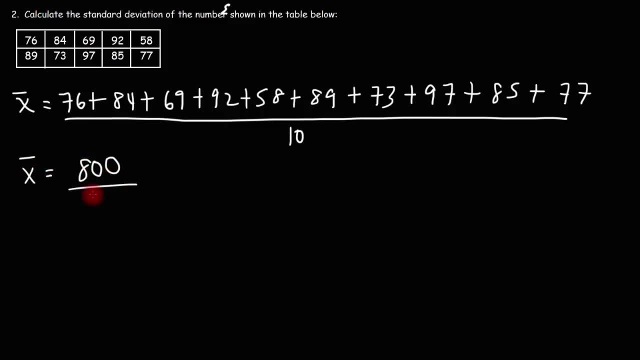 So the sum of those 10 numbers is 800. And if we divide it by 10, this will give us an average of 80. So that's the sample mean. Now let's calculate the standard deviation of the sample. So let's use the same formula that we. 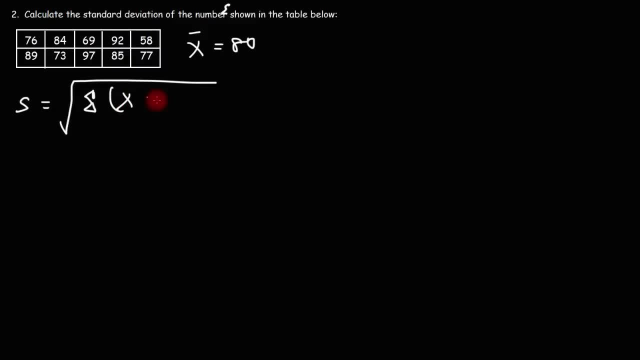 used earlier. So it's going to be the first number, 76.. Minus the mean, Which is 80.. And then squared, And then it's going to be the next one, Which is 84.. Minus the mean. 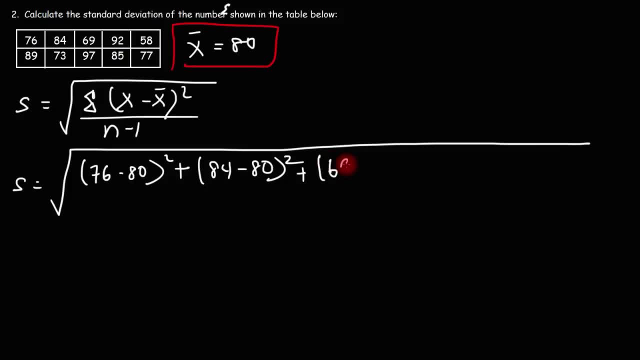 And then don't forget to square it. And then we need to do this for all of the numbers. So the last one is going to be 77 minus 80 squared, And then divide it by N minus 1. So we have 10 numbers. 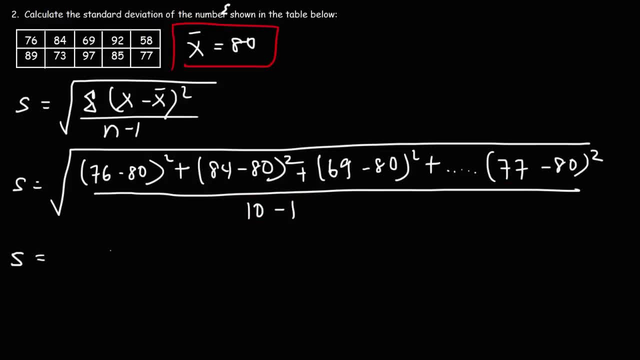 So this is going to be 10 minus 1.. Now, if you want to show all of your work without having to do so much writing, here's what you could do. So notice that we need to take the difference between each number and the mean. 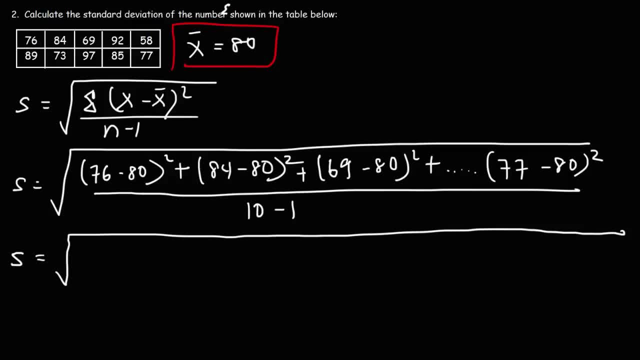 The difference between 76 and 80 is negative 4.. But when you square negative 4, it's going to be the same as square and positive 4. So we can simply write it as 4 squared The difference between 84 and 80. 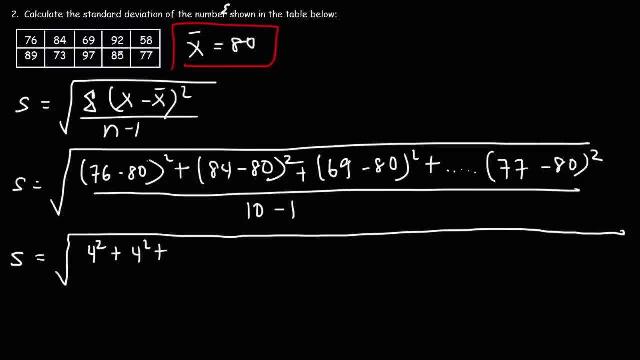 is also 4.. Plus another 4 squared 69 is 11 units away from 80.. The next number, 92,, that's 12 units away from 80. And then 58, if you do 80 minus 58, that's a difference of 22.. 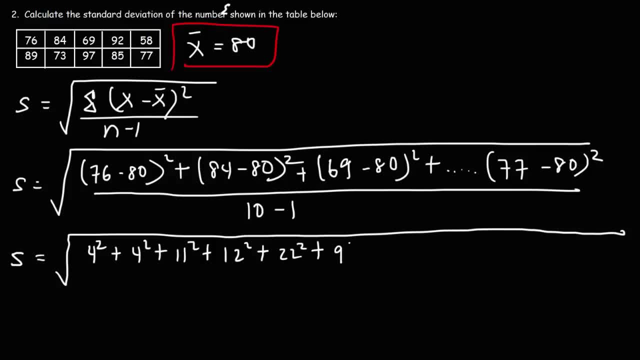 And then 89 minus 80, that's a difference of 9.. So you need to take the square differences of each number with the mean 73 minus 80, that's a difference of 7.. 97 minus 80 is 17.. 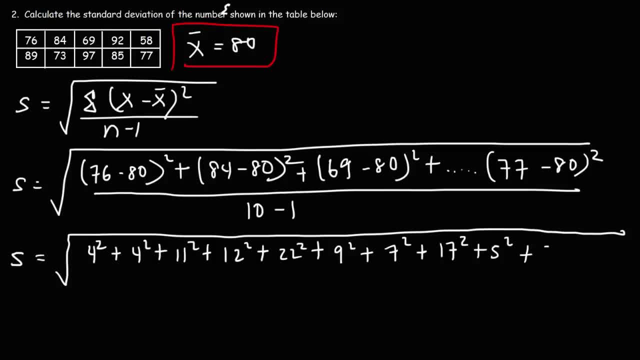 85 minus 80 is 5.. 77 minus 80 is 3.. Well, negative 3,, but we'll make it positive. 10 minus 1 is 9.. So now it's going to be easier to calculate it.